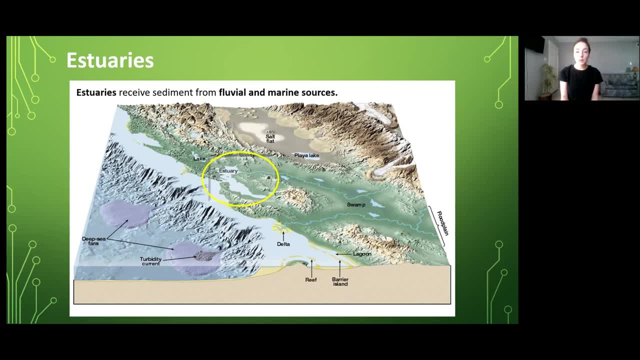 and marine sources and therefore this is going to be a large part of the discussion when we go over what kind of deposition is going to occur and what kind of stratigraphy we might expect in an estuarine sequence. So let's get into some background over estuary classification. 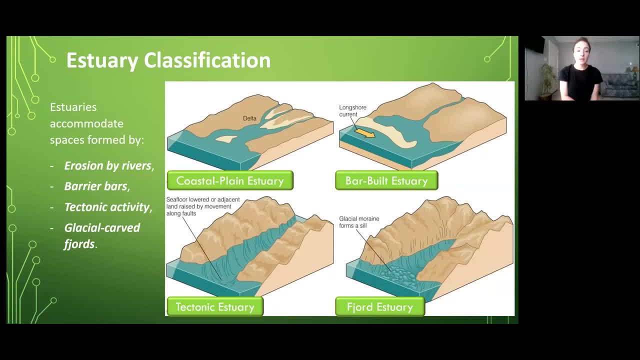 There are four different types of estuaries shown here in this figure. We have coastal plain estuaries, which are formed by erosion by rivers. Then we have bar-built estuaries, which are formed because of barrier bar formation, which is a wave-dominated system. 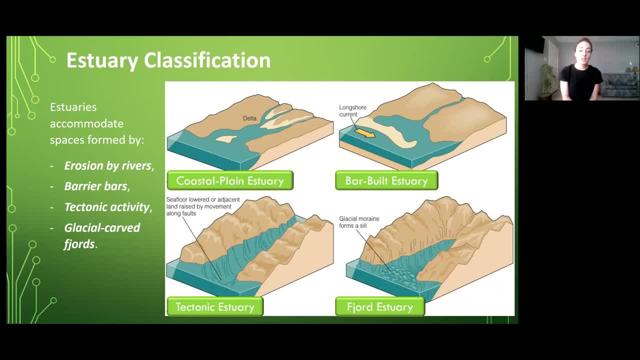 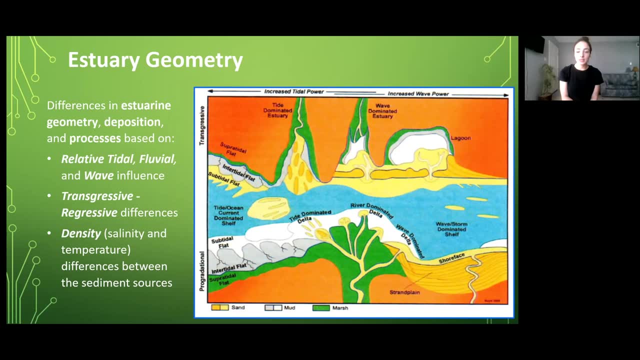 which we'll see in the next few slides. Then we have tectonically formed estuaries and then finally, glacially formed fjord estuaries, And the geometry, deposition and property of estuaries are different. So we're going to start with the estuaries. 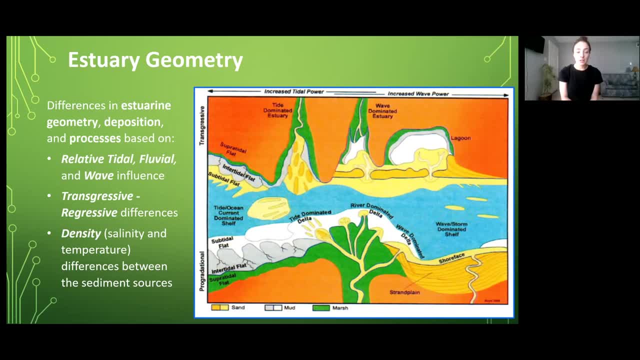 and then we're going to start with the estuaries. So we're going to start with the estuaries that occur in. estuaries is very dependent on the relative tidal, fluvial and wave influence. For example, on this figure we can see that, going from left to right, it goes from more. 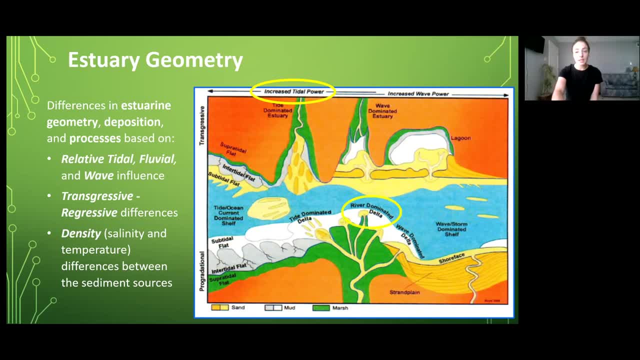 tidally dominated to the middle, which is fluvially dominated to more wave-dominated at the right. Additionally, the geometry processes and deposition in estuarine environments is also dependent on transgressive and regressive occurrences and we'll talk about this later in the 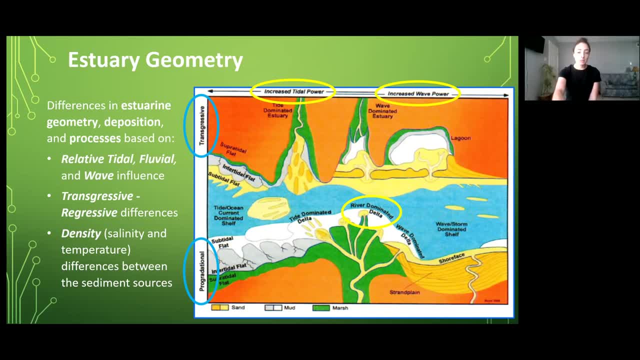 lecture, And then also density differences between the sediment source and the basin water, which we'll talk about also later in the lecture. So first let's talk about the geometry and what controls the geometry of estuaries. We can see that in this figure we have wave-dominated. 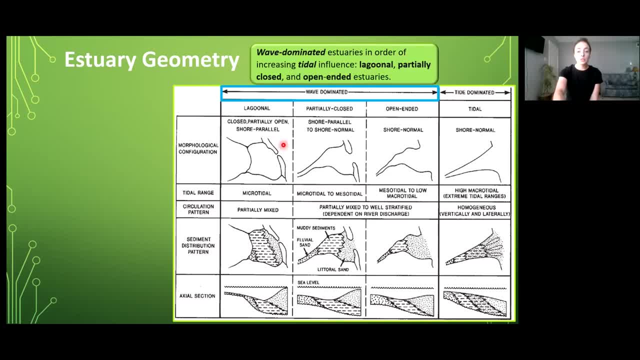 estuaries in the order of increasing tidal influence, going from lagoonal to partially closed, to open-ended estuaries, And then we have tide-dominated estuaries, called tidal estuaries. We can see that the geometry in wave-dominated estuaries is shore-parallel, whereas the geometry in tidal-dominated estuaries 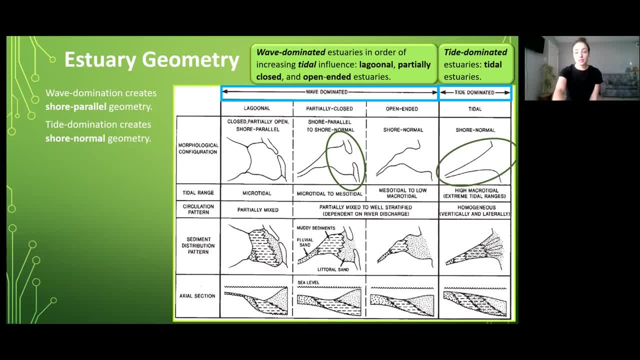 is shore-normal, so parallel to the shore rather than perpendicular or normal to the shore. Then we have the formation of bars. Wave-dominated systems form barrier bars by longshore currents, again distinguishing wave-dominated systems with that shore-parallel geometry. And then we have 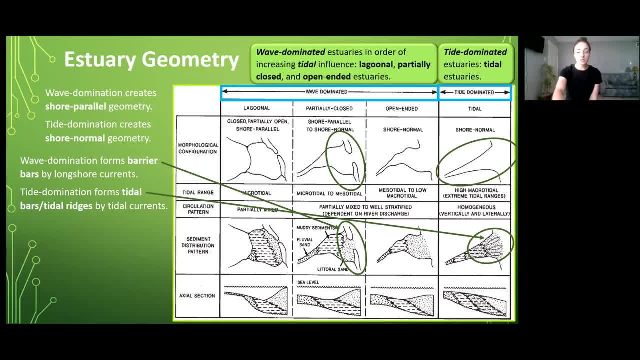 tide-dominated systems which form tidal bars and tidal ridges caused by tidal currents which, again, are normal or perpendicular to the shore. Lastly, for geometry, we have lagoons. Lagoons typically form when there is some sort of barrier bar, causing the accumulation of water behind it. 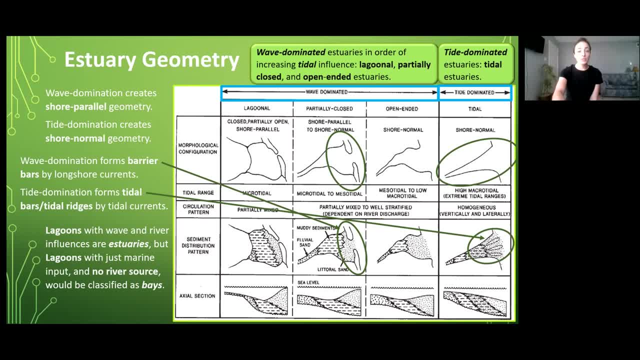 And in lagoons they can either be fed by marine and fluvial sources or just marine. When lagoons are fed by both fluvial and marine sources, we call these lagoons. However, when lagoons are fed, 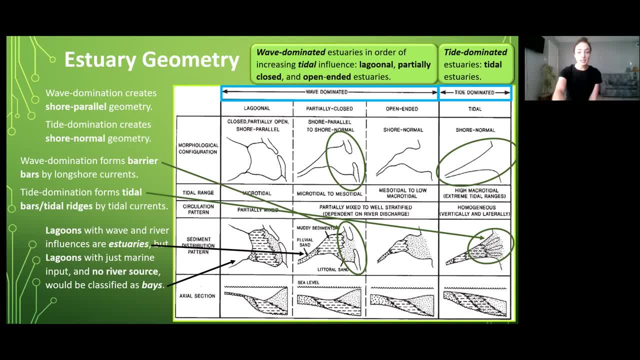 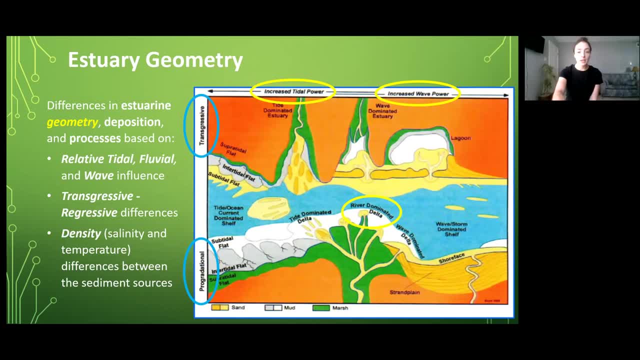 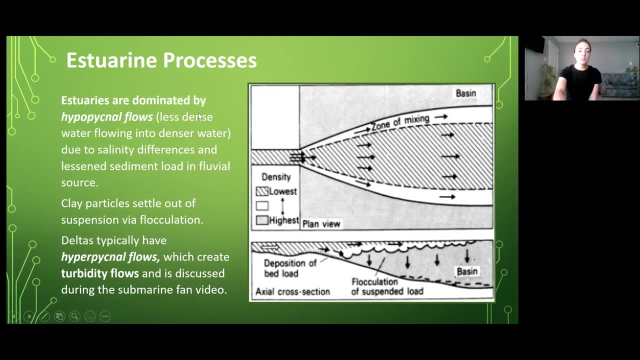 by marine sources only, with no river source, these are technically classified as bays. So now that we have that classification, terminology and geometry out of the way, let's get into the deposition and processes in estuarine systems, Like we talked about previously. we mentioned 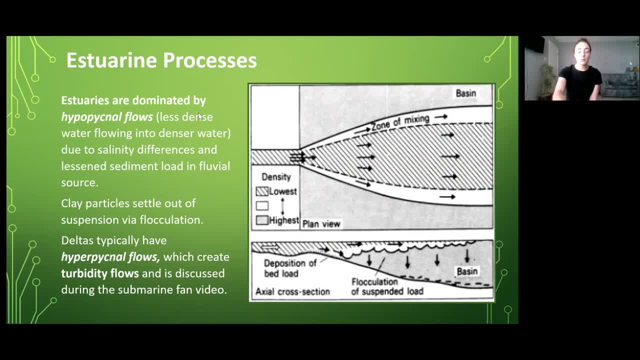 that the density of the inflow versus the basin of water will influence the deposition in estuary environments. Luckily, there's only one flow type that is typical of estuarine environments, and other environments, like deltas, differ greatly. This makes it easy to distinguish estuaries from 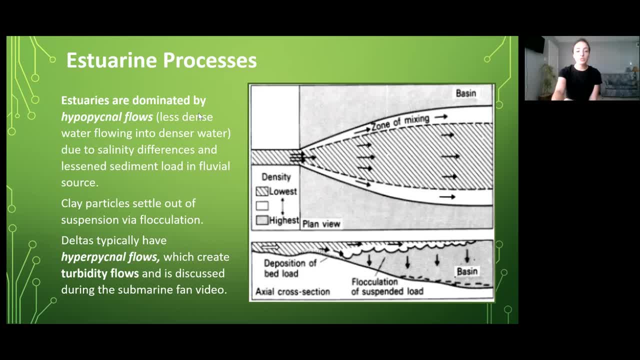 other depositional systems. So let's get into the deposition and processes in estuarine systems. In the rock record, for example, estuaries are dominated by hypopicknall flows. Hypopicknall flows are flows where less dense water flows into a denser water body. This is typically caused 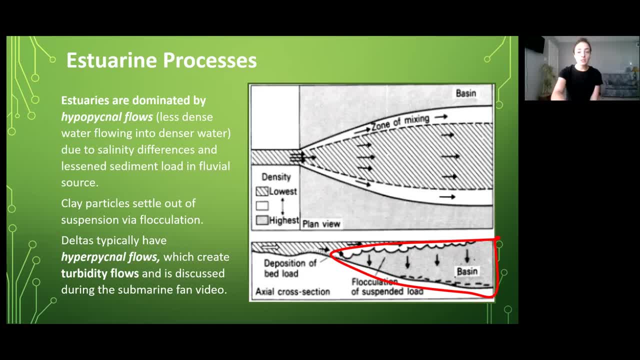 because the salinity in estuarine basins is greater than the fluvial inflow because of the marine influence. However, where fluvial inflow is dominant and you have deltas forming and building out further offshore due to progradation, these are typically dominated by hyperpicknall flows. 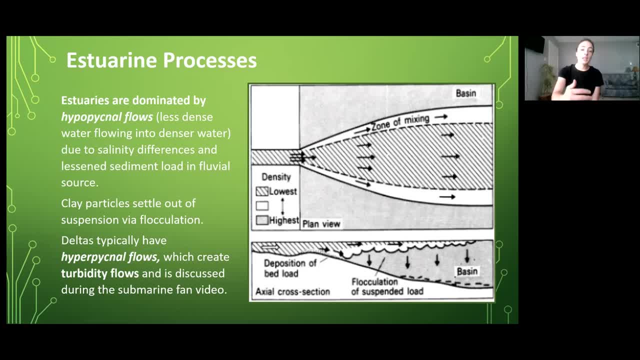 These hyperpicknall flows are flows in which the incoming flow is more dense than the water it is flowing into. This is typically because the fluvial source has a high sediment load and this causes turbidity flows, which will be discussed in the submarine fan video. Additionally, I discuss more. 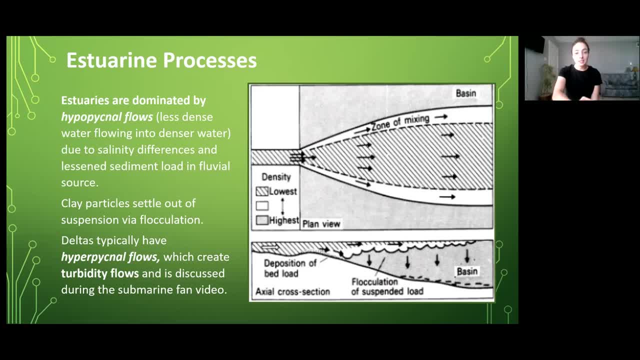 about deltas and the processes behind delta deposition in the deltas video And lastly, if you want to go back and look at the lacustrine video, you can learn a little bit more about the deposition and sedimentary structures that form due to the flow of sediment. So let's get into the 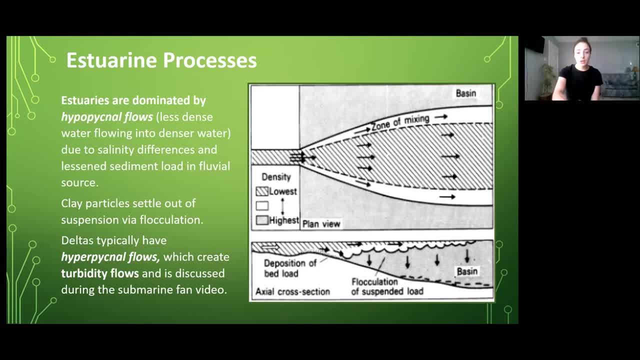 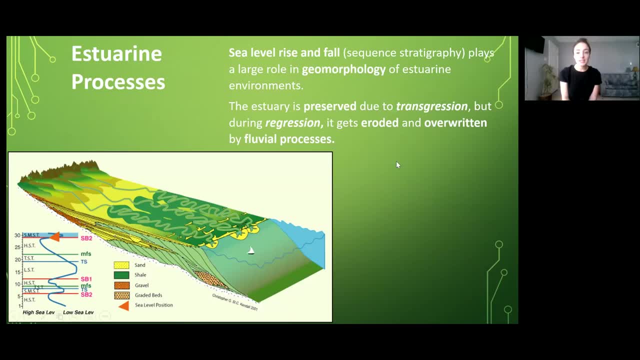 different types of inflow events: hypo, hyper and homo picknall flows. But for this video, let's move on to how sea level affects estuarine deposition. Sea level rise and fall can play a large role in determining the geomorphology of estuarine systems. The estuary is preserved due 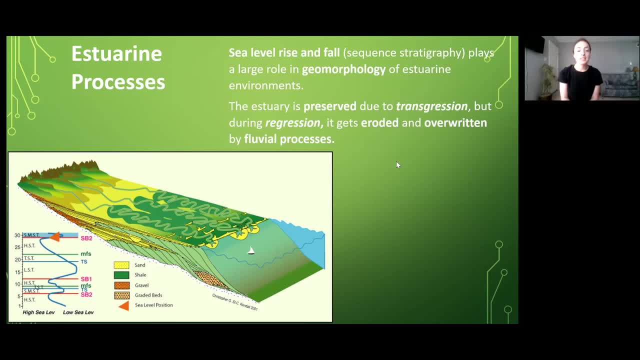 to transgression, but during regression gets eroded because it is overwritten by fluvial processes. To show this, we have this figure to the bottom left. What we can see is this is during the shoreline moves further inland, as opposed to a regression when the shoreline moves further. 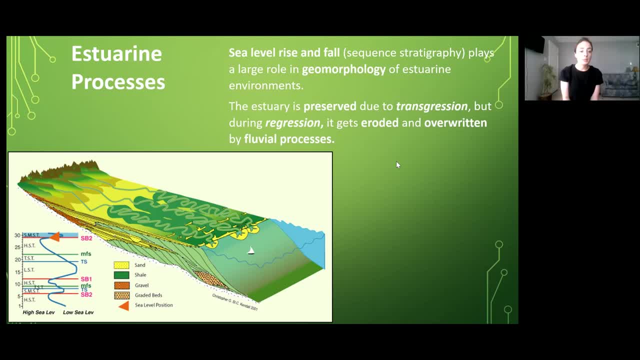 basinward, The shoreline moving further inland or transgression can be due to a rise in sea level, And when the sea level rises, we get this wonderful estuary environment to form, if all of the marine, fluvial and tidal influences are balanced to where an estuary would be formed. However, when we get 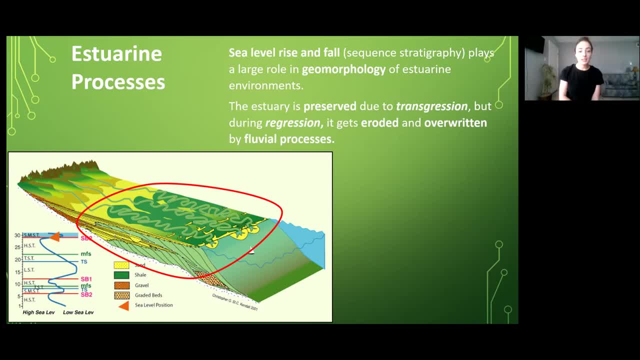 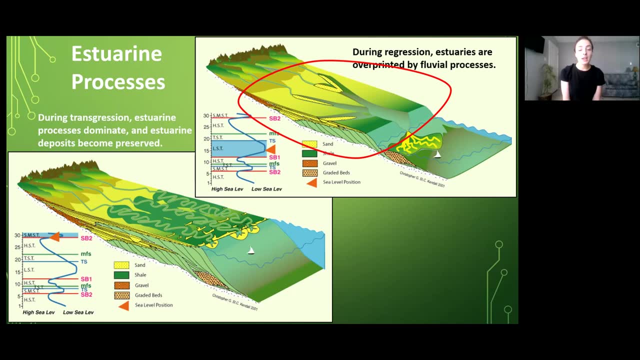 regression occurring after this transgressive sequence. we see fluvial processes overprinting a lot of the estuarine deposition. So when we get a rise in sea level, we get this wonderful estuary deposition. This is why we know that estuarine deposition and preservation dominates during. 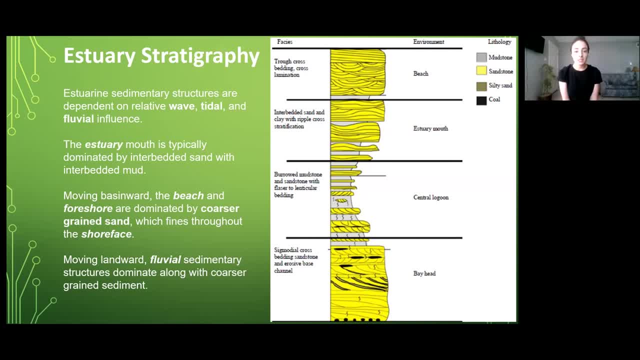 transgressive events. Now let's talk about estuary stratigraphy. We've talked about the geometry, the processes, the deposition, but what about when we walk up to that outcrop? What are we going to see to make us know that this was an estuary environment? This is a strat column showing 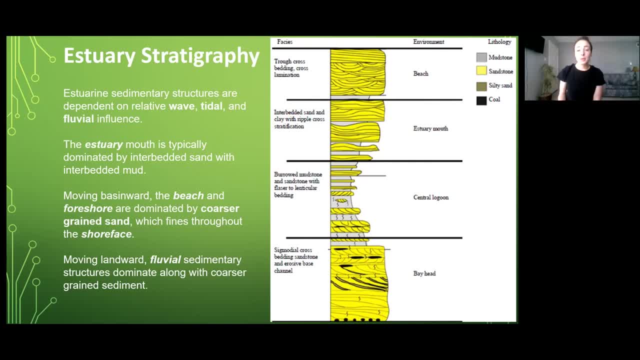 showing the progression from further onshore, from the bayhead to the central lagoon, to the estuary mouth, to further offshore, to the beach, etc. We already mentioned that estuarine processes and deposition are dependent on relative wave, tidal and fluvial influence. 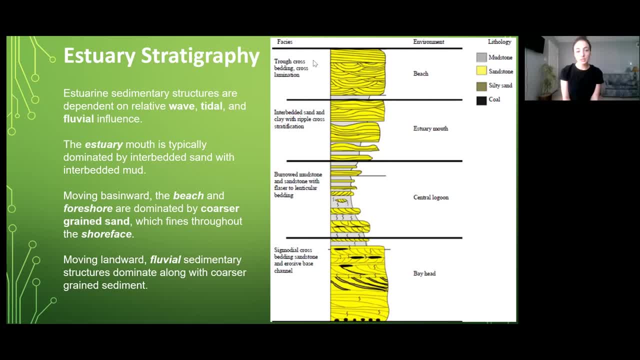 This is also true for the sedimentary structures in an estuarine sequence. The estuary itself is dominated by interbedded sand and mud faces, and as you move to the beach and the foreshore you get coarser-grained sand which finds throughout the shore face further offshore. 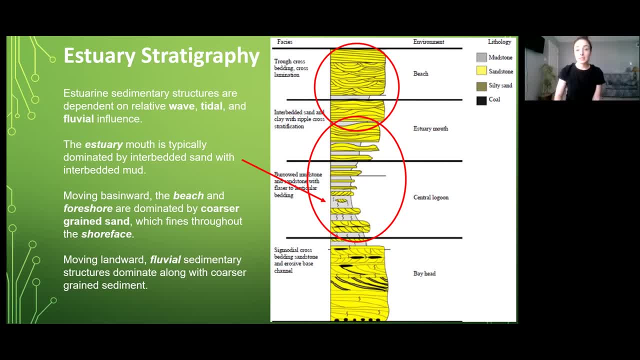 Then moving landward back, moving away from the ocean basin and estuary, you get fluvial sedimentary structures along with coarser-grained sedimentary structures. This is also true for 你能在 Haus, nicht im eisen ini放. Beatrice was the.